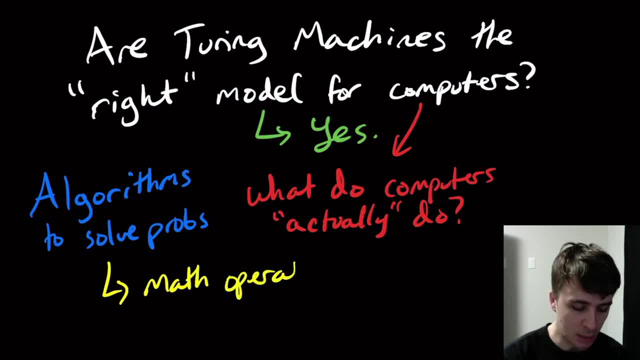 of math operations of some kind, Like multiplying things or adding one for a program counter or storing things somewhere in some memory. So it's some kind of math operation happening all over the place. So the question about whether the right model is: can Turing machines actually do math stuff? 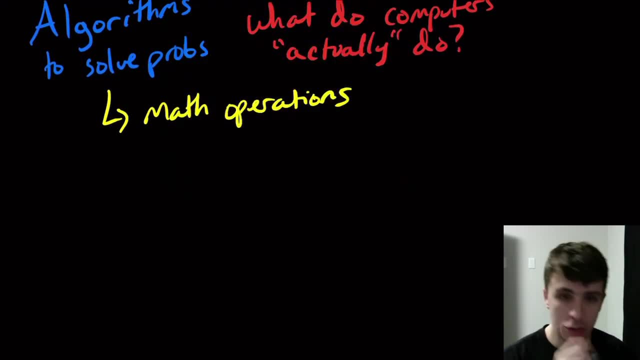 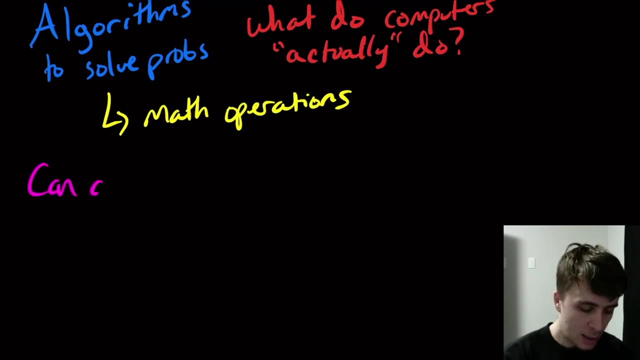 And the answer is actually yes. So what I want to convince you is that we can do all of these operations pretty easily. Can a Turing machine take an input number- can't spell number, that's troubling X- and write X plus one on the tape. So like the simplest possible operation is adding one to the to a. 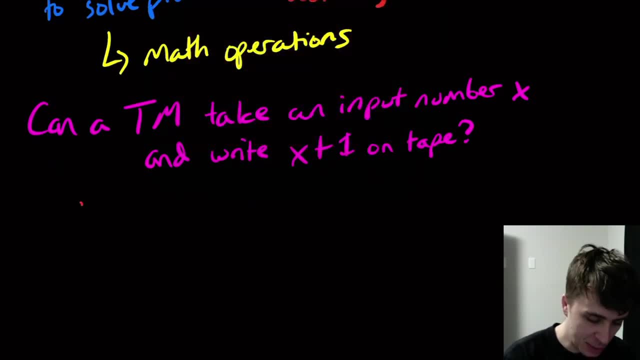 number. So let's just look at this as an example. So let's say we have zero one one, zero one one, So this is just some number. Then the normal way we add one to this is: we want to add one. 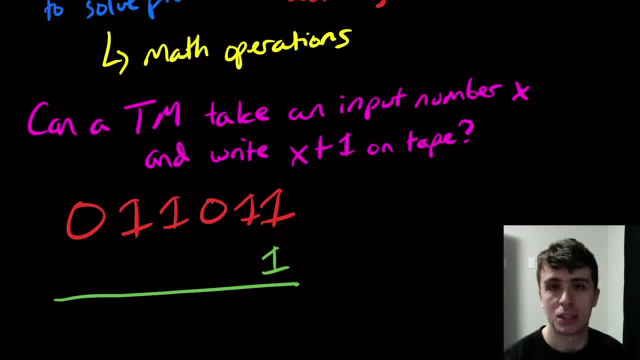 So we look at this, right here we see two ones. So we're going to write down a zero for the result and then carry a one over to the next column And then so that we have a one with the carry up here, So we have a one right here in the number. So we're again going to get a zero and carry a one over to. 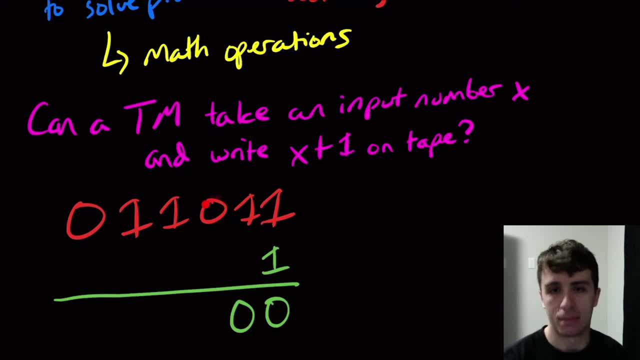 here. So we have a one in the carry and the zero which is in the number. So we'll have a one downstairs, because that's what zero plus one is and there is no carry as a result. So because there's no carry, we're going to have the rest of the number just copied and pasted. So the real way. 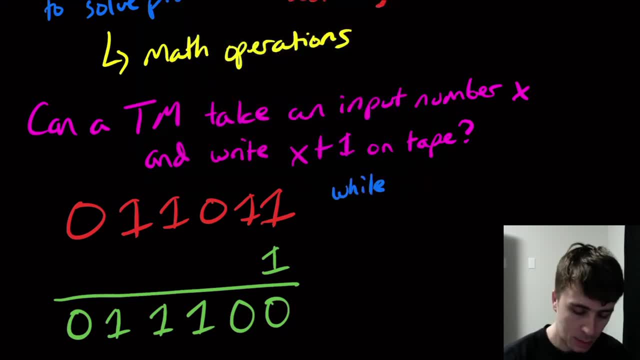 of doing this is to while there is a 1 at the end, although actually that's not the right phrasing of this. so what we should actually do is start from the end and going to the front, so from the end of the, the right side of the number, to 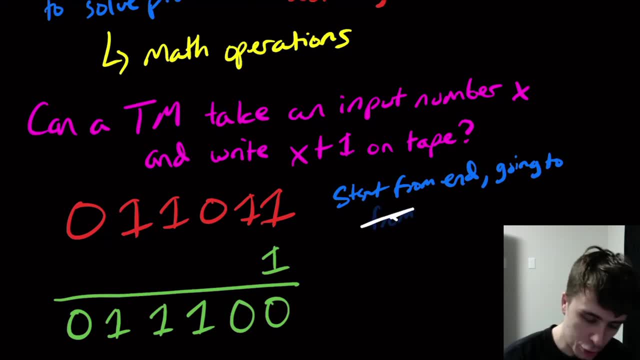 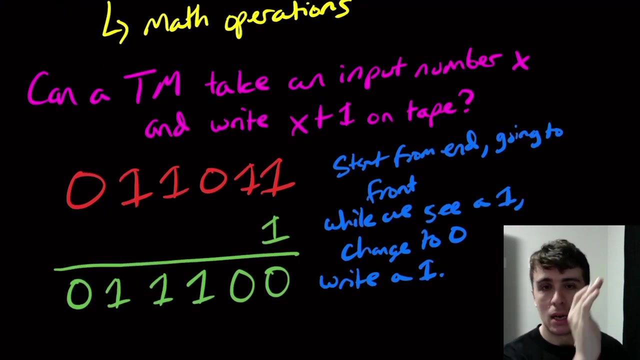 the left going to the front and while we see a 1, change to a 0, and then at the end we write a 1, once we're done with that. So when we're done seeing 1s and changing them to a 0 in the result we're going to at. 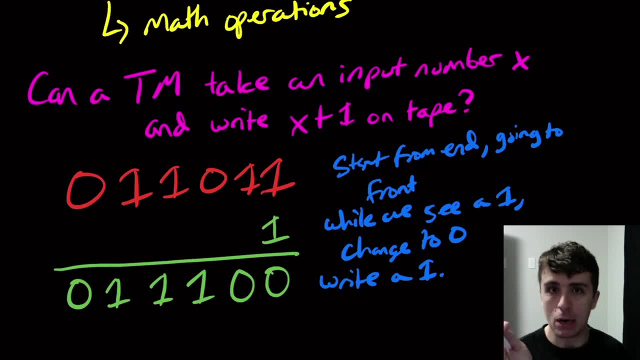 the very end, change it either. if it's a 0,, we're going to change it to a 1, but if the entire number was all 1s, then by adding 1, we're going to make the number slightly larger by one digit, longer, one bit longer. So we're going to put a 1 on the. 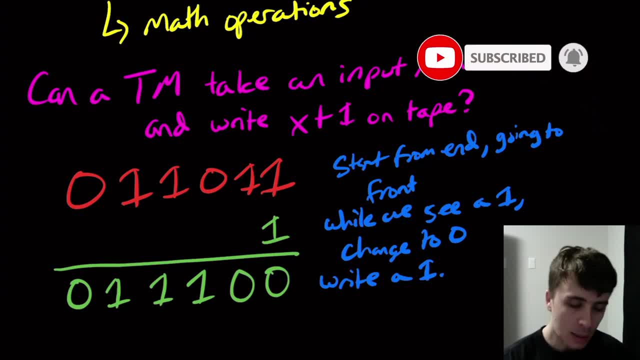 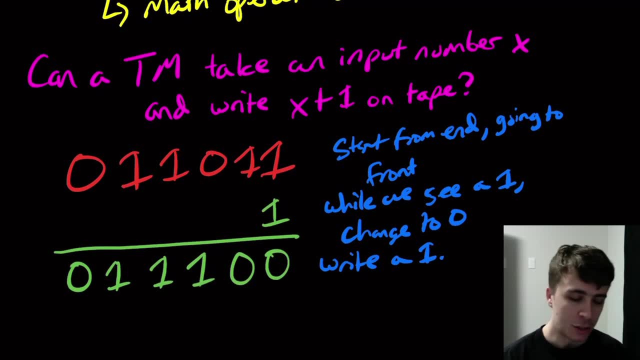 front of it, and that's pretty easy to do. Okay, so then in that case, it would be 1 with a bunch of 0s after it, which is exactly what we would expect anyway. Okay, so we can actually have a Turing machine, take an input number and increment it. 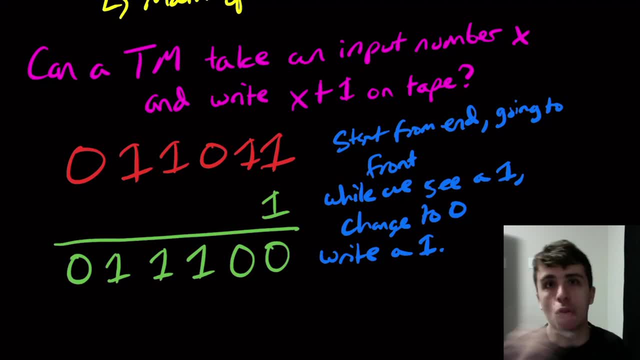 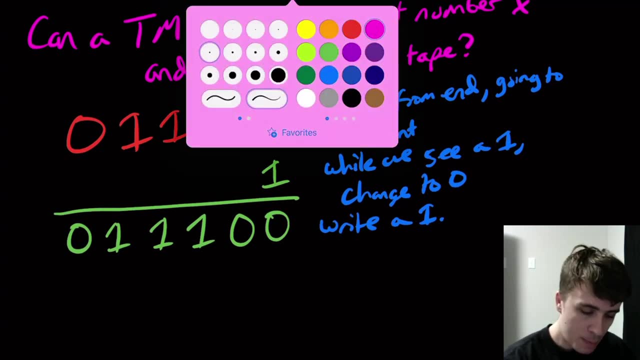 to 94, we're going to like write it by 1, so 0s must not be anymore than 1, then we're going to want everything 1s, because that is everything initial. Then we can just 산: That's pretty much it. that would work perfectly. And then 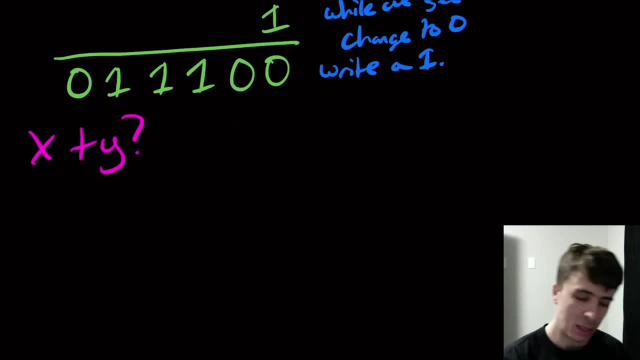 once everything's Tambien, we can actually change. the've been pretty good. Okay, so we can figure out this one and we need 0s, and what we're going to do is this: we're going to give one a number for and we're going to take all 1s of k2c2,. 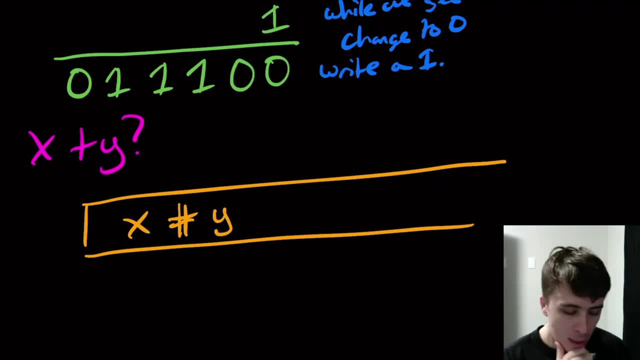 again. So there's no confusion here. And how would we actually write? let's say, I want at the very end there to be x plus y over here. So I don't care what's in these two parts right here, I care just to have x plus y written somewhere. So how do we actually handle? 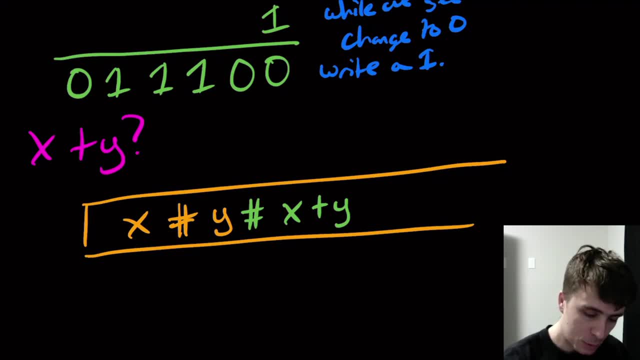 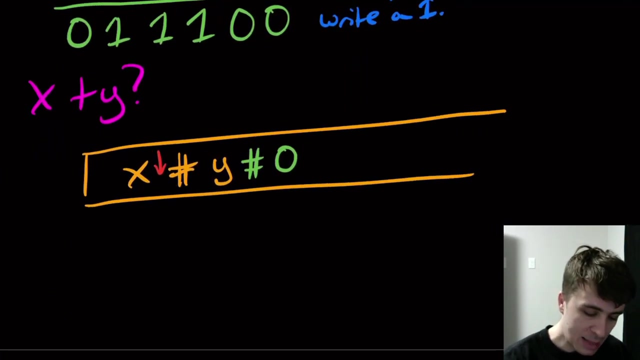 this. Well, the trick is to initially start this with 0 right here, because we haven't done anything. And then what we're going to do is we're going to subtract 1 from x, And subtraction works very, very analogously to adding by 1.. And at the same time, we're going to add 1 to y. 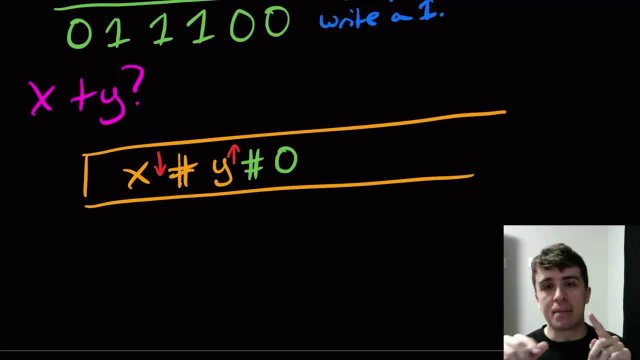 So x plus y is the same thing as taking 1 away from x and adding 1 to y and then adding those two together, because the minus 1 and the plus 1 cancel. So what we're going to do is we're going. 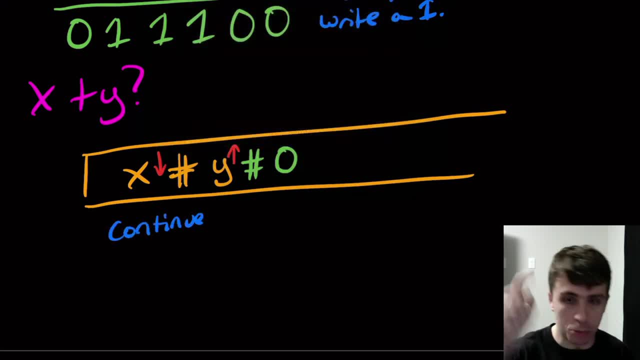 to continue this process, subtracting 1 from x and adding 1 to y, not touching that third one yet, until x is equal to 0. And so, at the end of the day, what happens is that we're going to have 0 over here. 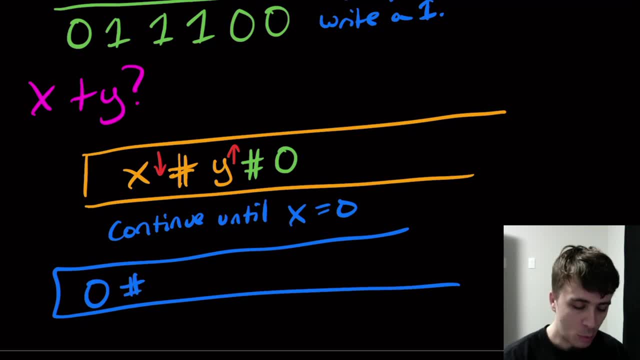 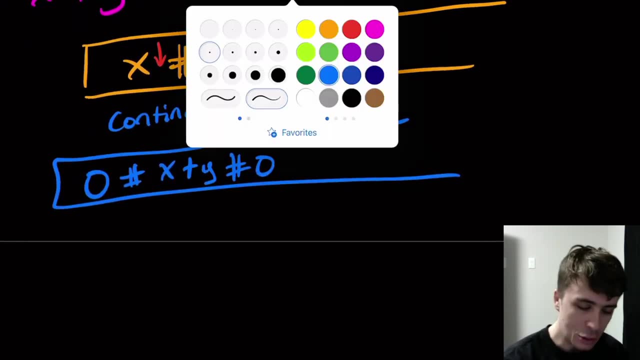 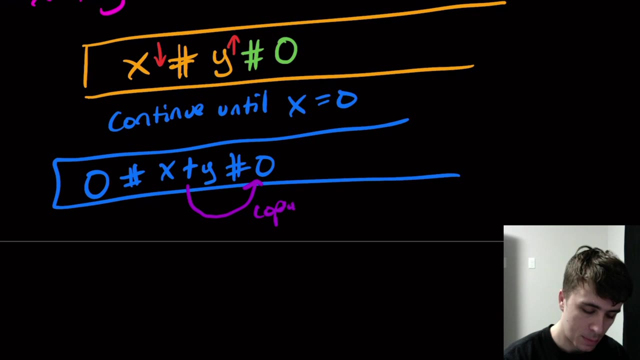 because we're going to continue until we get there. Then we're going to have equivalently x plus y here and then a 0. And then all that I need to do- which is really easy- is just to copy and paste this over to here. So, copy plus paste, And in fact, 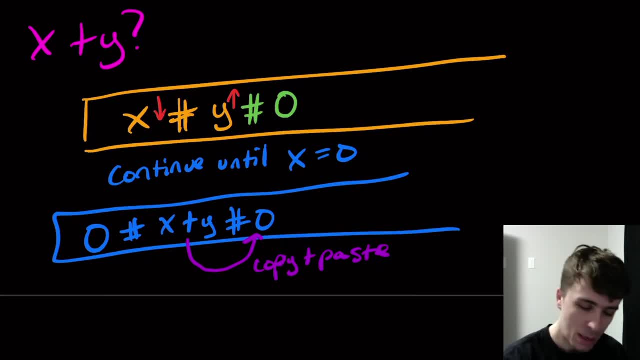 if we didn't care where the x plus y was on the tape, then we're already done Because it's right here. But if we didn't want it here, we would have to copy and paste, And that's easy to do And I invite you to actually think about how we do that, But it's pretty easy. 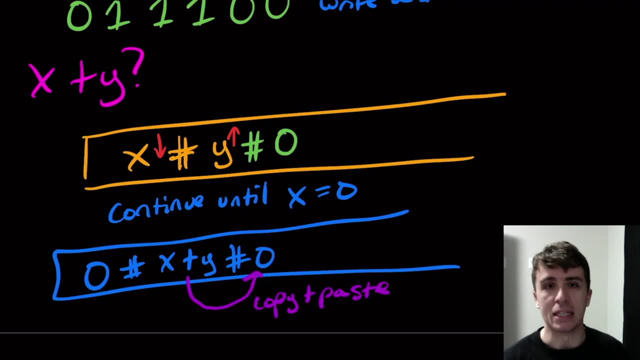 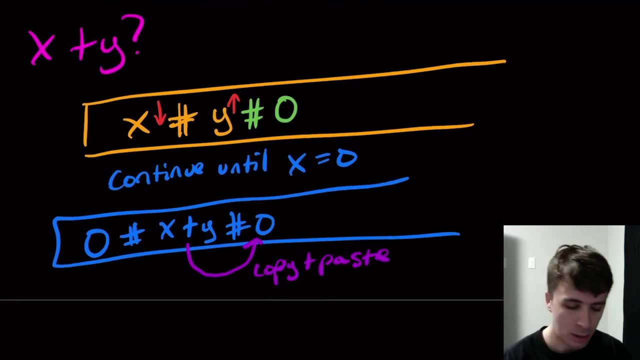 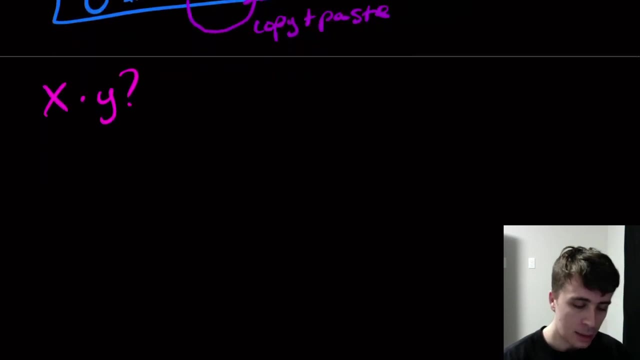 to do. OK, So we can add two numbers pretty easily, because all we need to do is to subtract 1 from 1 and add 1 to the other one in tandem with each other until one of them becomes 0.. What if we wanted to do x times y? Then what we would need to do is: 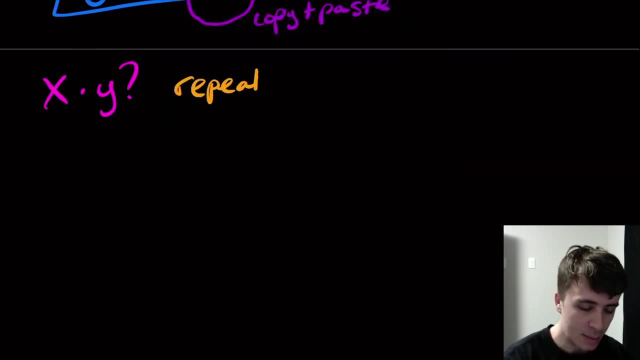 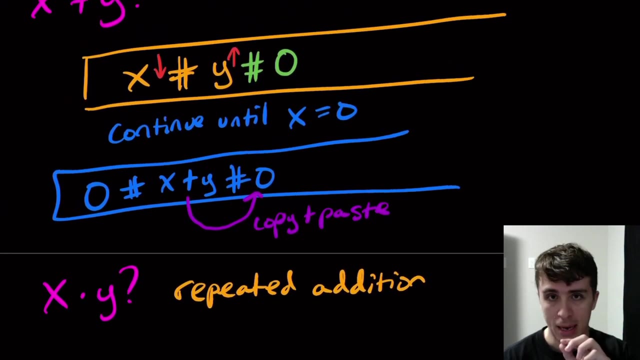 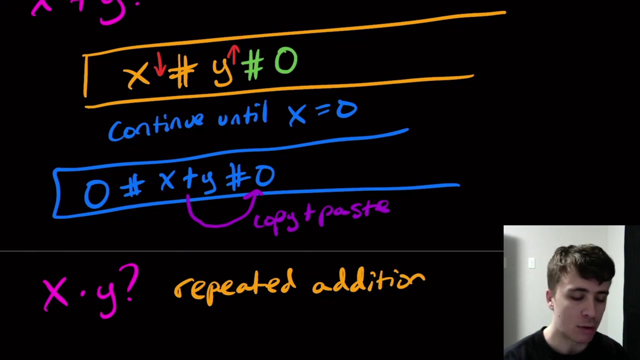 instead of subtracting 1 from x and adding 1 to y, what you should do is subtract 1 from x and add the original x in whole to y, In whole to y, So it's not just 1 and 1 here. 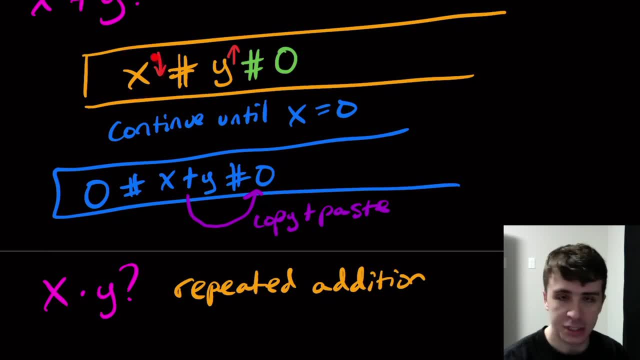 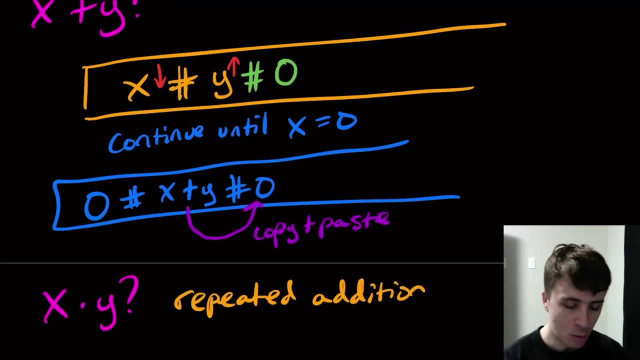 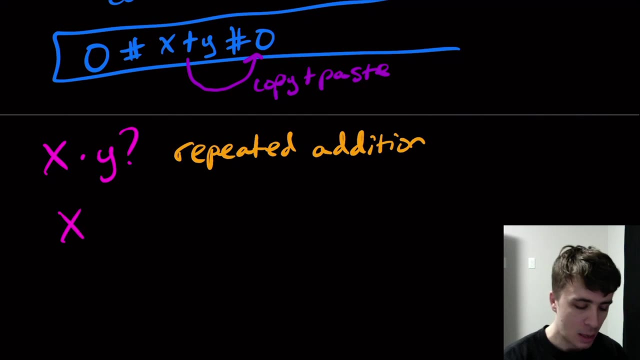 it's 1 and a whole x right here. This number is changing, but the thing we add to y is always going to be exactly the same. OK, So that will allow us to do repeated addition and get x times y in almost identically the same way. What about x to the power y? Then that is just repeated multiplication. 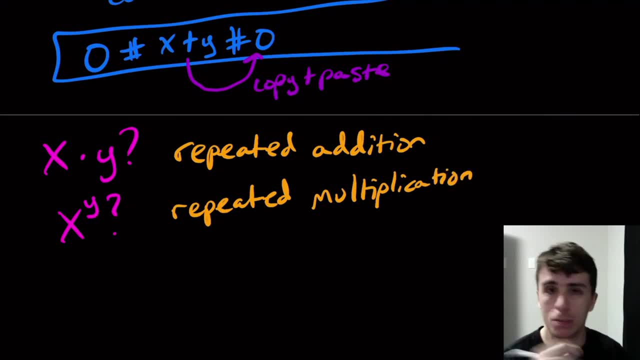 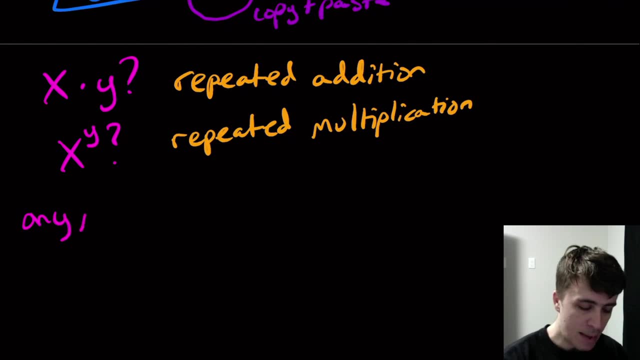 Almost identically, And I want you to think about how you do that too, But it's almost the same idea. What if we wanted to do any math operation done on a computer? Then what you can notice is that it's just going to be some finite combination of multiplies. 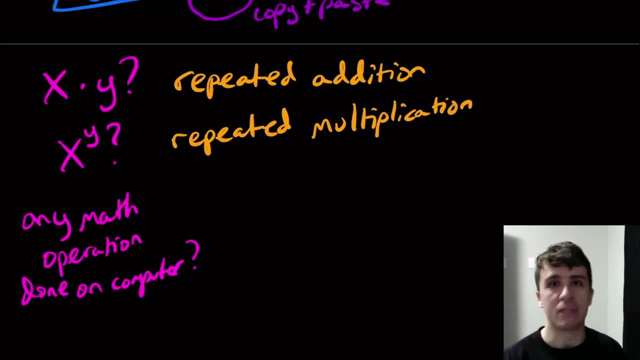 additions, subtractions, even divisions, And I invite you to think about how the division works here. It's just going to be a finite number of these operations, So I'm not going to worry about something like, say, cosine of x, because in that case it could be an irrational output. 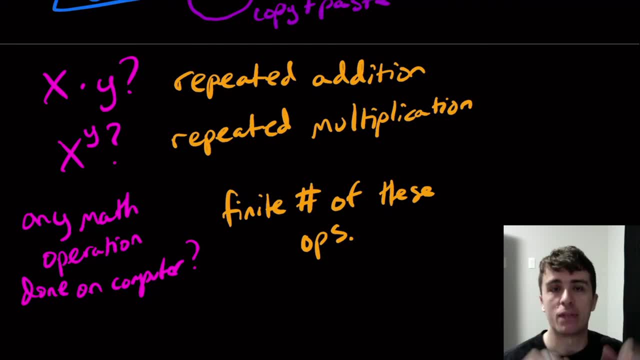 and it's impossible to write a finite length representation of that. I'm worried about what an actual computer does, And an actual computer doesn't write down an irrational number. It may work with it in some different kind of representation, But it's still working with binary numbers here which involve addition, multiplication. 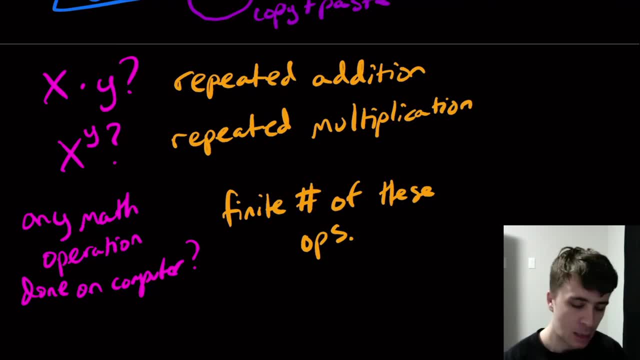 subtraction and division and powers. So, in fact, if it's just a finite number of these, then we can write an algorithm and the Turing machine could effectively do it, as long as it's a finite number, And it always is, because we don't do an infinite amount of. 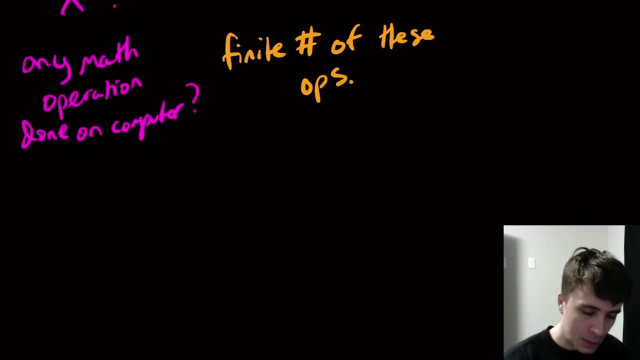 work in a finite amount of time. Okay, So what was noticed is that these two mathematicians, Church and Turing- I'm not sure if they did it together, but this is attributed to them- And in fact, there's a third mathematician I don't remember who's taken off this list for some. 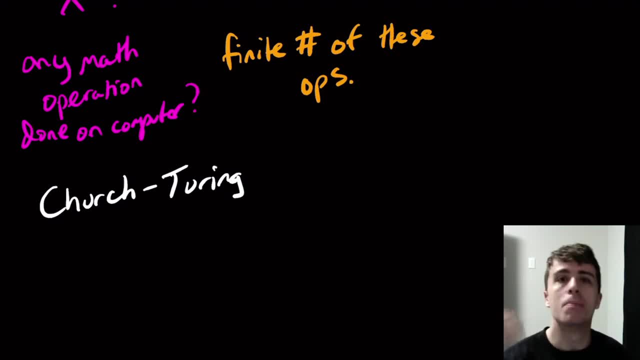 reason. But it's not just these two, but this is what is proposed, something called a Church-Turing thesis. So it's not something that you can prove, but it's just something that is true anyway, but is just not provable. So what they? 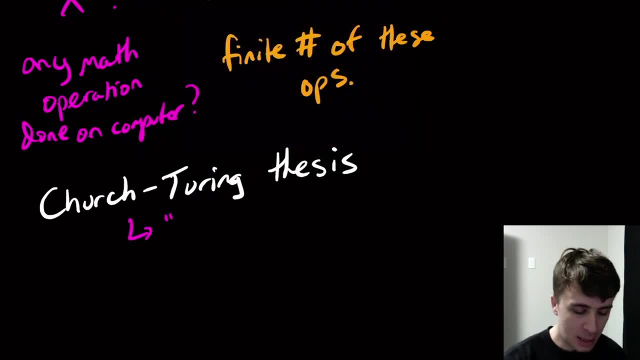 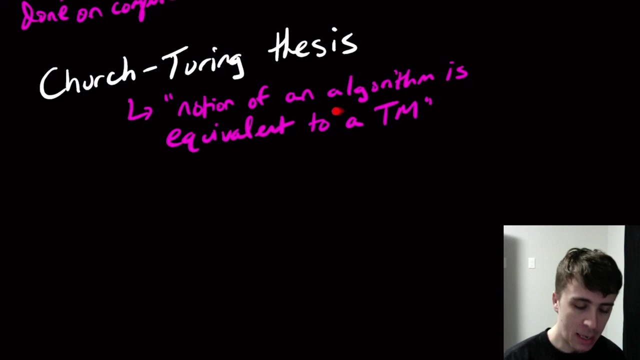 effectively said? is that any? Actually, I should say it this way: The notion of an algorithm is equivalent to a Turing machine. Okay, And this is actually pretty profound. We actually kind of did half of it already, which is So. the notion of an algorithm is that if we have any algorithm, then I can make, And by algorithm. 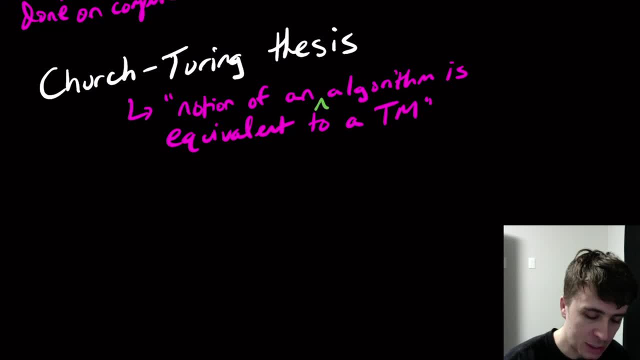 I mean an intuitive algorithm. So this is an important word here. So intuitive: Any kind of intuition about what an algorithm is, what you believe an algorithm to be. that's effectively what a Turing machine is, Or we can convert it into a Turing machine, And 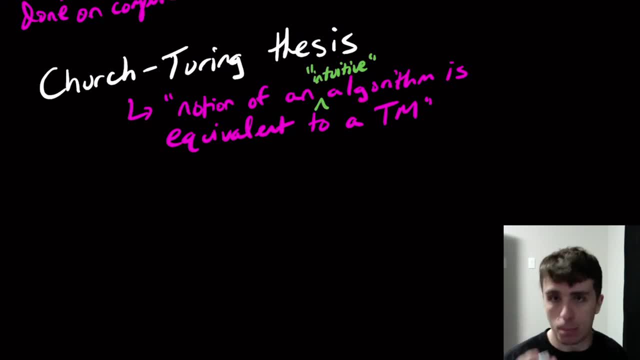 here we have shown that if you have the modern notion of what an algorithm is, then you can convert it to a Turing machine And, conversely, if we can actually build a Turing machine simulator- and many people have done so and I invite you to actually write a Turing machine- 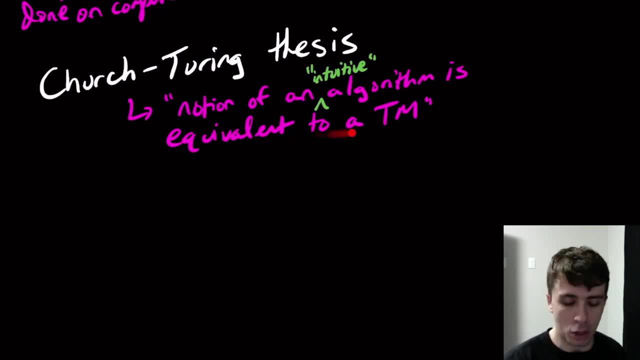 simulator on your computer. So take a Turing machine as input and simulate it. So, because we can convert an algorithm into a Turing machine and a Turing machine into an algorithm. that's going to create a difference. So you have this idea and you can actually use the concept of the shoulders on the entire machine to create your algorithm, Right? 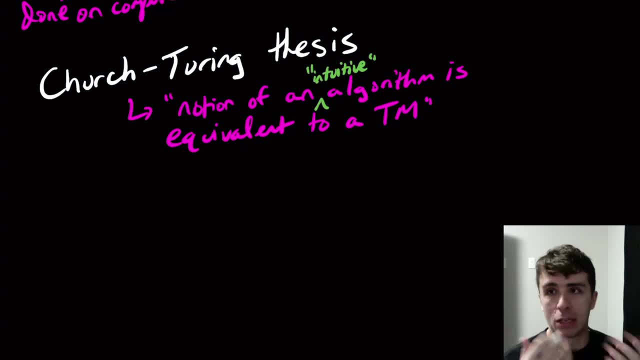 into an algorithm, because we can just simulate the Turing machine. Therefore, we can actually say that Turing machines are equivalent. So it is true, but the only issue with this and being able to actually write this as like a theorem or something is that I need then to define for you. 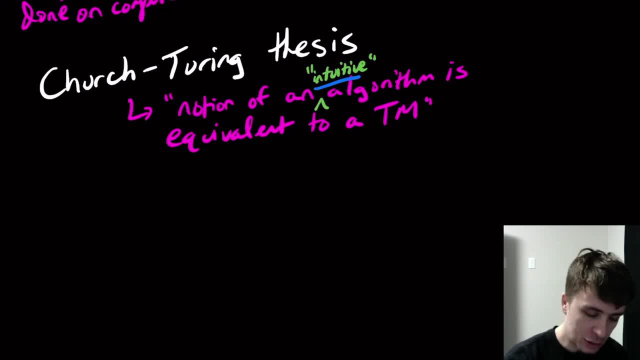 what intuitive actually means, So does intuitive intuitive. does that mean we only work with, say, the x86 instruction set? Does that mean we work with all possible instructions, Because then there could be some weird instruction that we have no idea how to do? 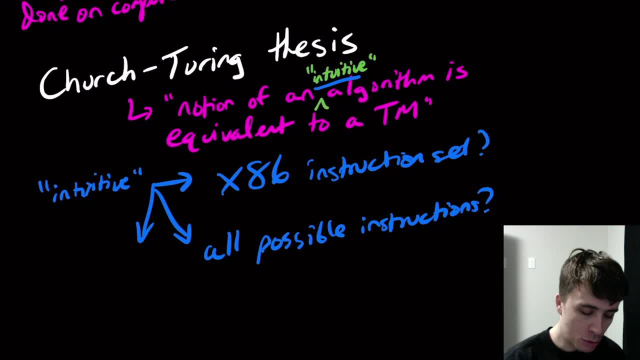 but it's still an instruction. Do we do all instructions? It could be all instructions Except not except all instructions done in a finite number of steps. Because so this kind of fixes this thing, because maybe there's an instruction, that's just impossible. 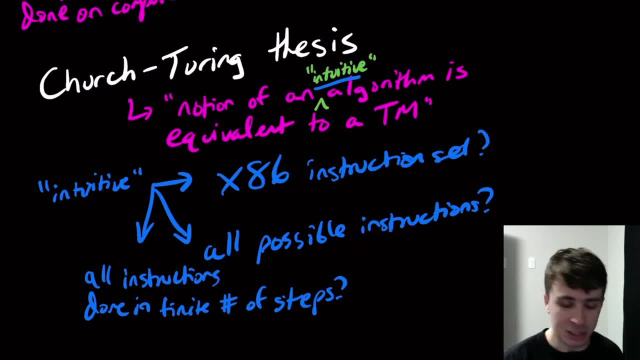 to do in a finite amount of time, but it would be included in this list. So maybe we only focus on the ones that only take a finite amount of time, And so it just really depends on what intuitive means, And if I define for you what intuitive means, then we could effectively prove this. But 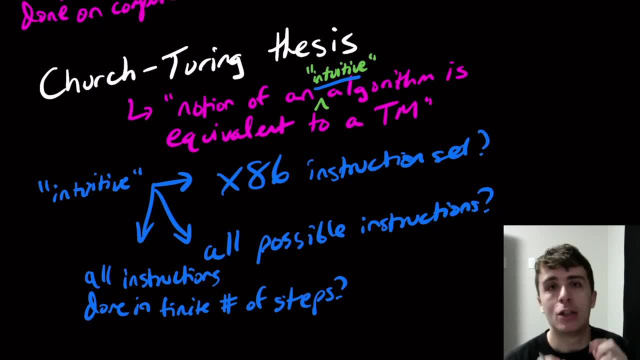 there's no outset to what intuitive actually means, But that's what they proposed- is that, even though that this statement is true for modern computers, we can't actually prove this. So the logical consequence of this- because it's true- is: if an, not an, if a problem. 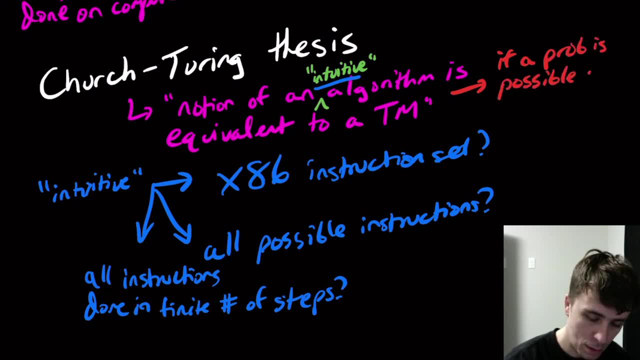 is possible with a Turing machine, then we can solve it with computers, right, Because they're equivalent. If I can do it with a Turing machine, then I can just do a conversion and make and I have an algorithm that I can run on an actual computer. But here's the important consequence. 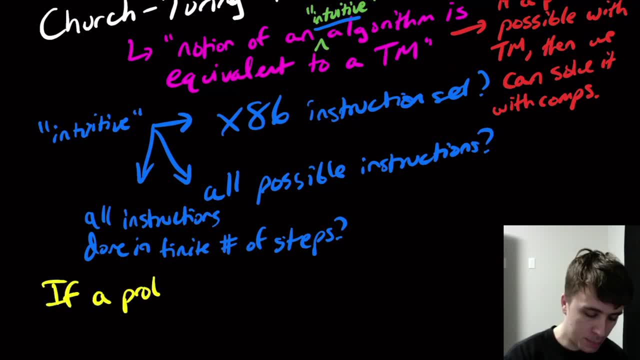 So if a problem can't be done on a Turing machine, then no computer can solve it. I'm not saying that the Turing machine, the computer, has to be really, really fast And the Turing machine is slow. In fact the Turing machine is almost always going to be super slow. but I'm saying: can it be done? 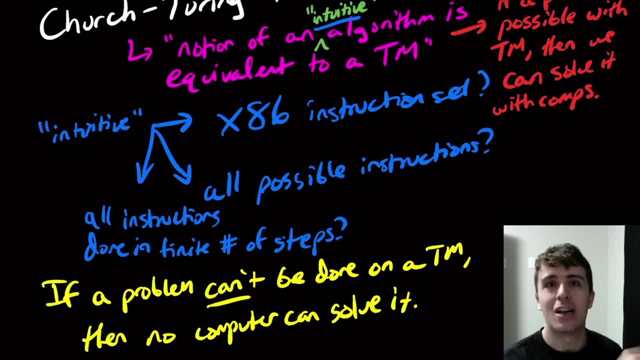 at all. And if it can't be done, how can anyone do it? Nominee이고 lige be done at all on a Turing machine, then no computer, in any amount of time, can solve it, because they're equivalent to each other. So we're going to be using these facts constantly.